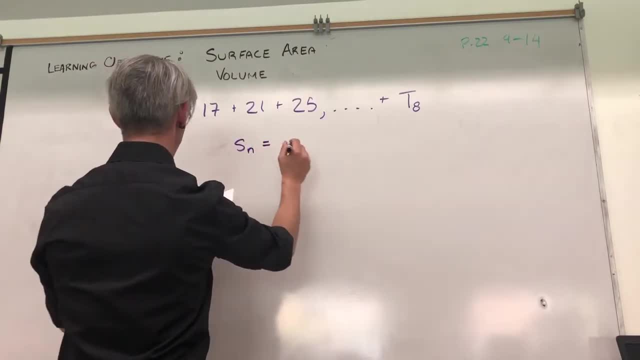 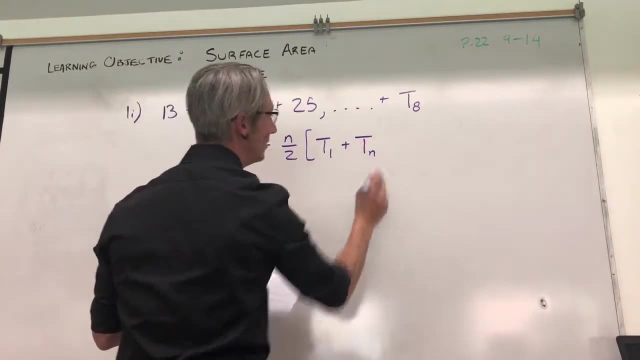 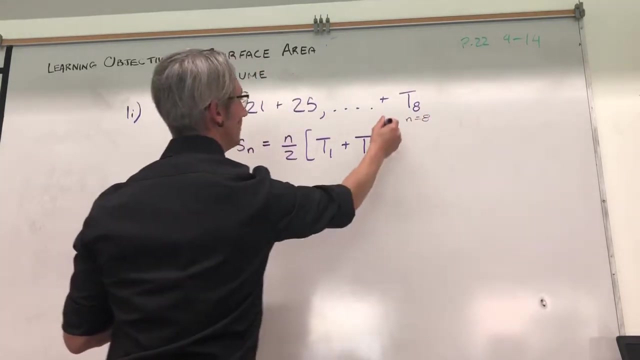 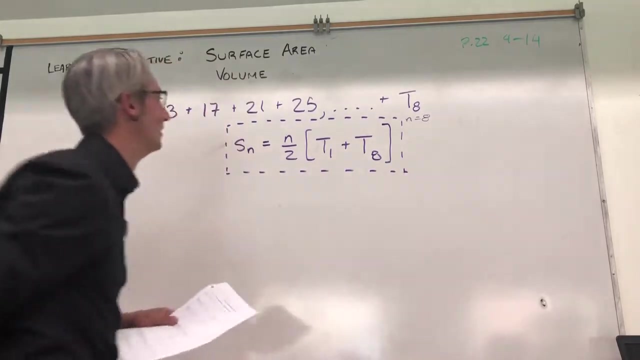 The first one that they give us is: SN is equal to N divided by 2, multiplied by the fourth, The first term plus the last term, TN. or we could write T8, because we know we go all the way to T8.. Okay, So this is, that is my equation And I need to know. so I know N. 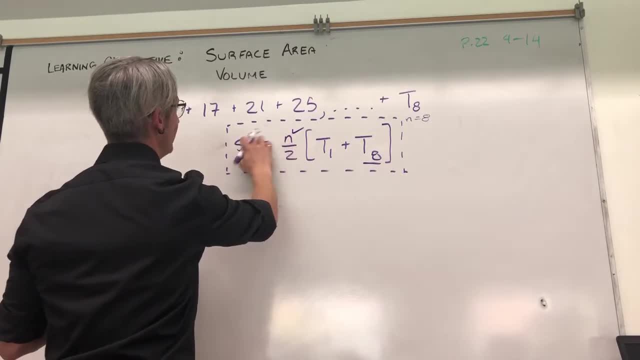 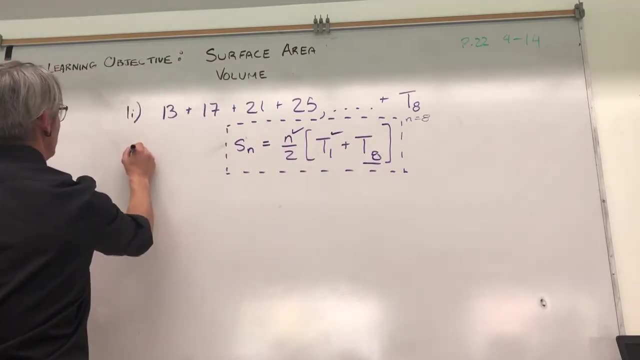 I know N is 8.. I know SN. I don't know SN, sorry, And I need to know. so I need to know, I don't know, and I know T1, but I don't know T8. So I know T1 is 13.. D: I know we're. 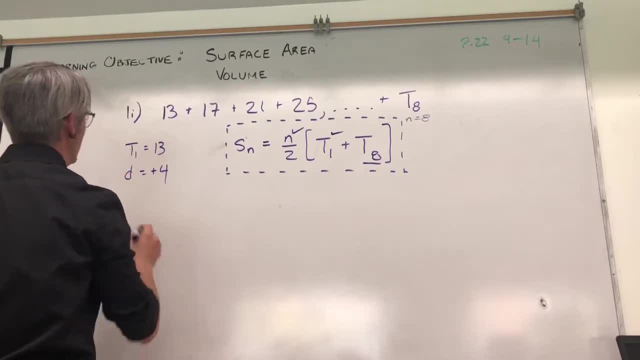 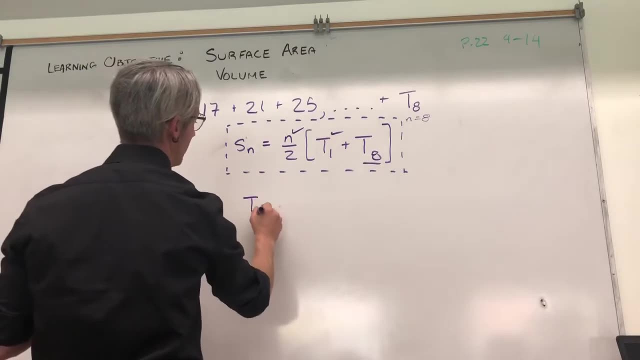 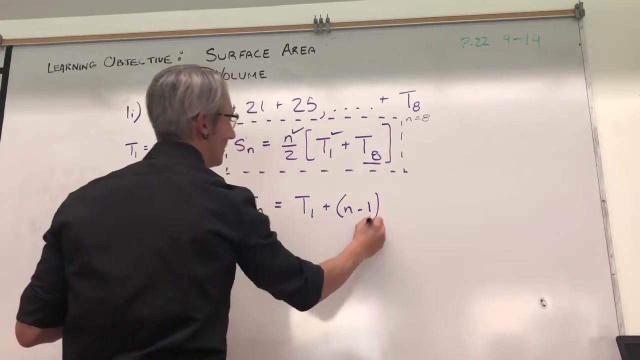 going up by plus 4 every time, And TN or T8, I don't know. So I have to use my formula for TN, which, if we go back, is T1 plus N minus 1 times D. Okay, we're cool. Okay, we're cool. 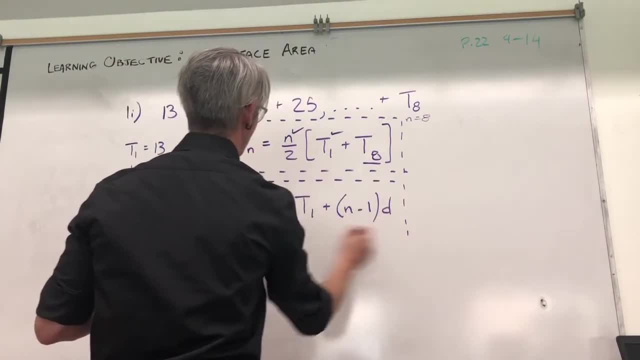 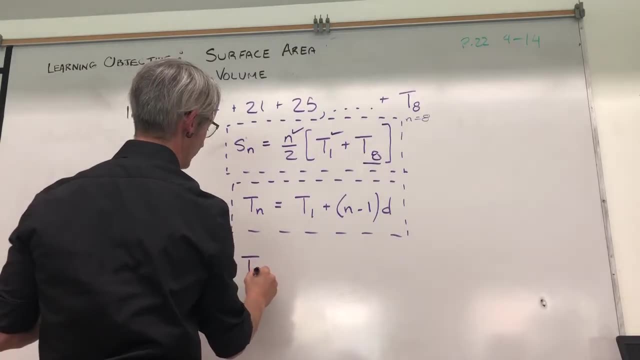 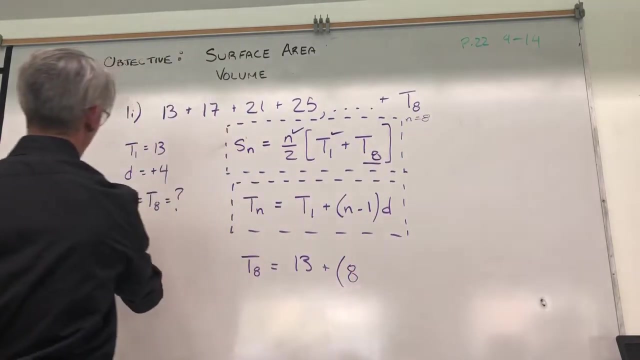 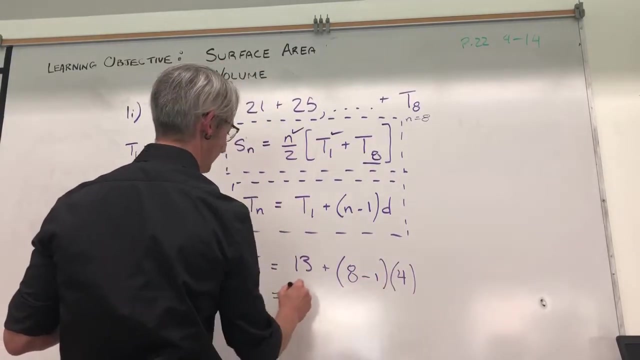 So this is 21 over 2.. So in order to use this formula, I need to know what TN or T8 is. Okay, So I do this. Is 13 plus N is equal to 8,, 8 minus 1 times 4.. Is 13 plus 7 times 4.. So 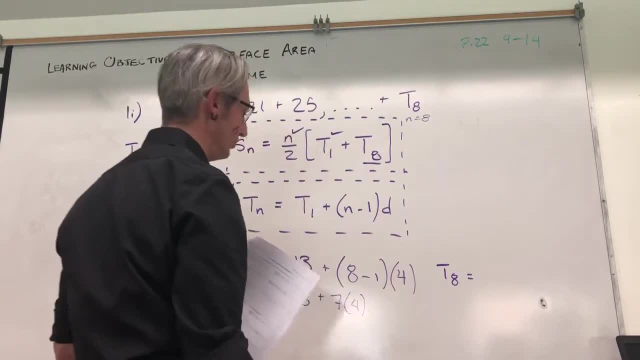 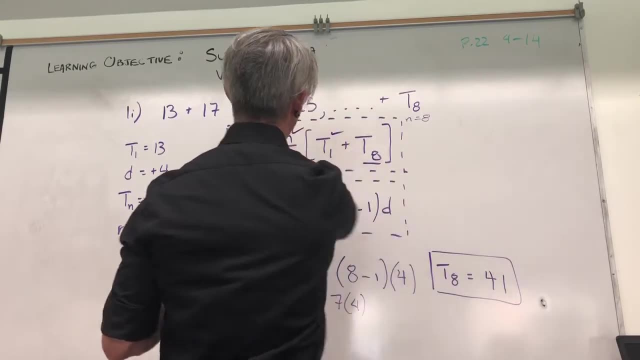 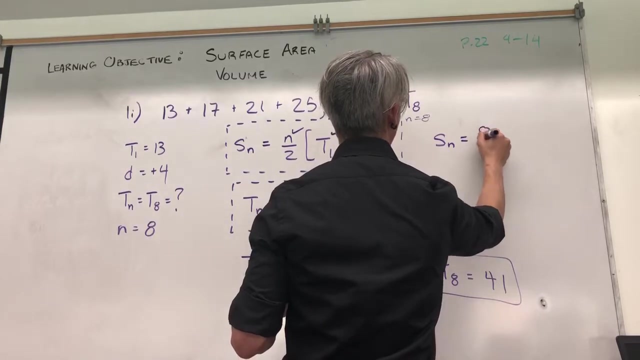 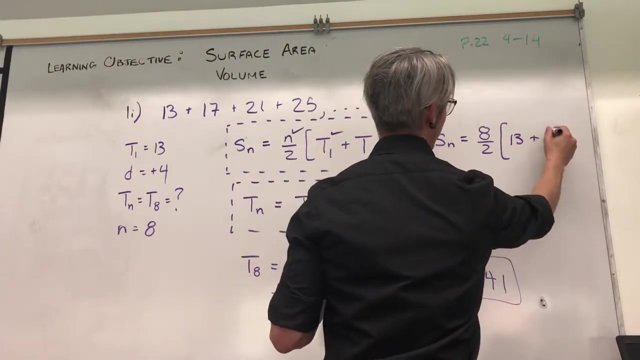 T8 is equal to 13 plus 28,, 41. Okay, I'm going to take this and now I can use SN there. So SN is equal to 8 divided by 2,, 13,, which is T1,, plus T8, which is 41. Okay, SN is equal. 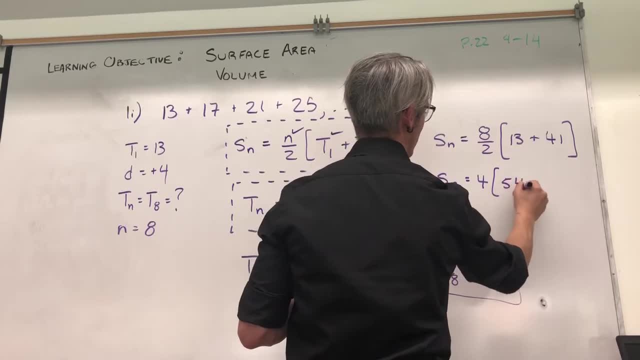 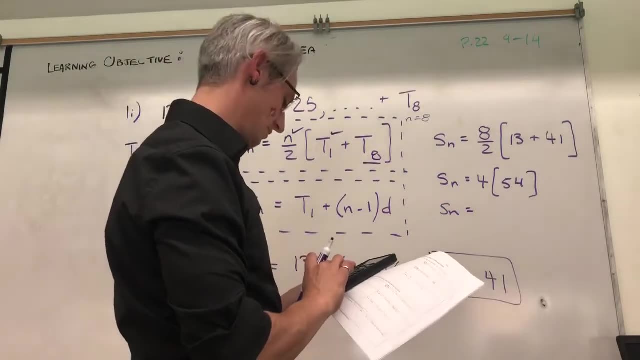 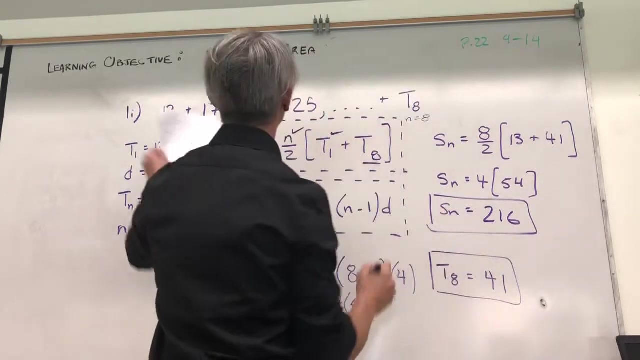 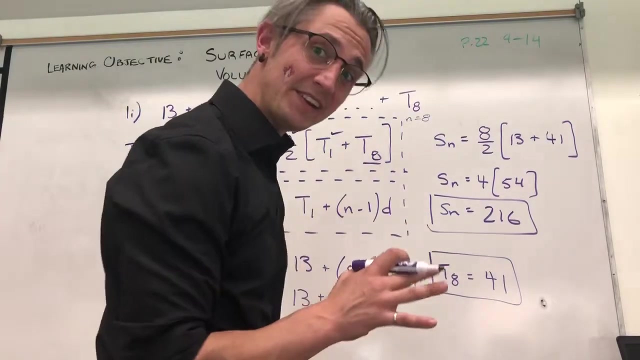 to 4 times 54.. SN is equal to 54 times 4, 260.. So the sum of this 8-term series is 216.. Okay, If I went too fast, you can rewind it now. Yay, Okay, Let's move on, shall we? 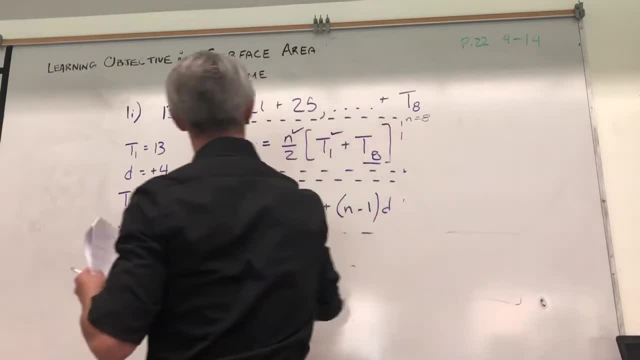 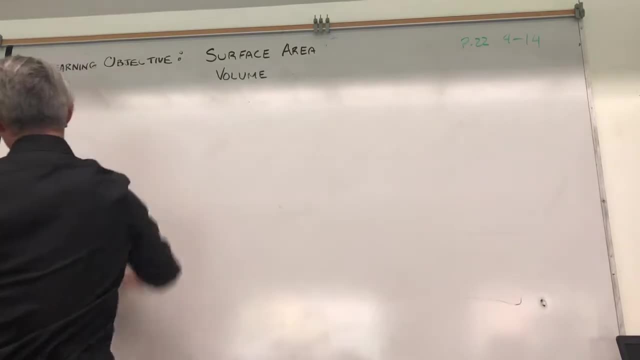 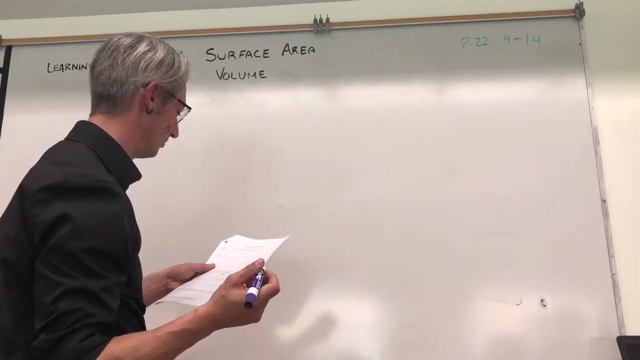 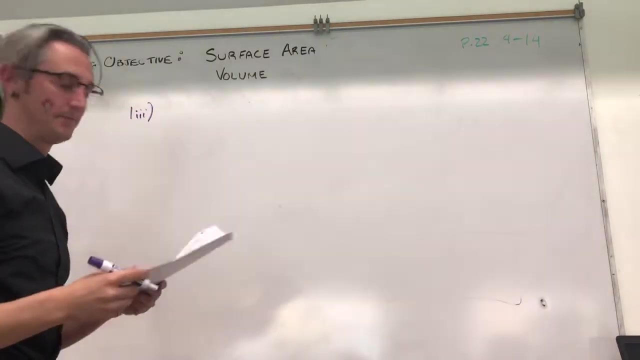 Let's do: hmm, Okay, let's do 4, 1-4.. Or we'll do 1-3.. 3-I, We'll do 3-I. Okay, So I've got 9 plus 14 plus 9.. So I've got 9 plus 14 plus 9.. So I've got 9 plus 14 plus 9.. So 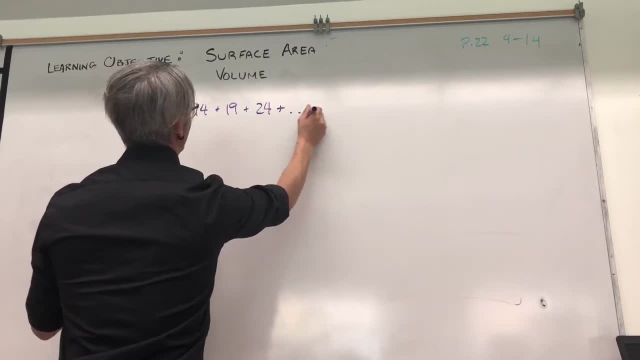 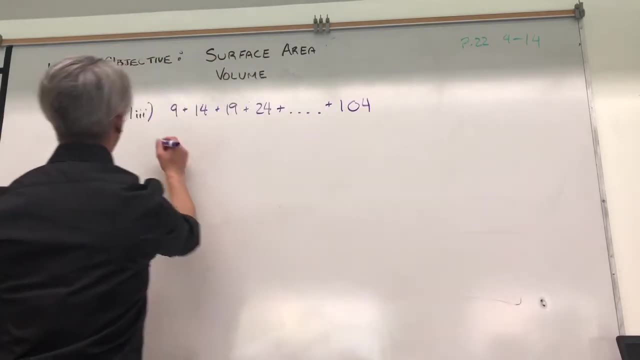 I've got 19 plus 24, plus all the way to plus 104.. Okay, So I'm looking at this and my T1, I know, is 9.. My difference is plus 5.. I know that my N-th term, I don't know what. 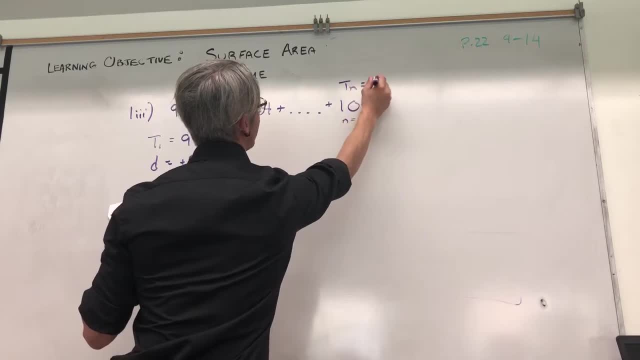 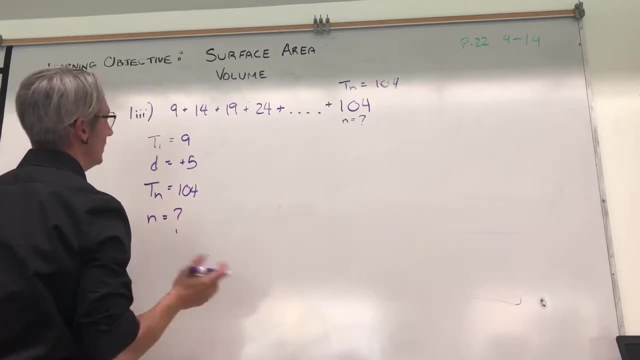 N is, but I know that the last term is 104.. So TN is 104.. I don't know what N is, So I don't know anything else I need. I don't know, So I'll go to my first equation. SN is equal. 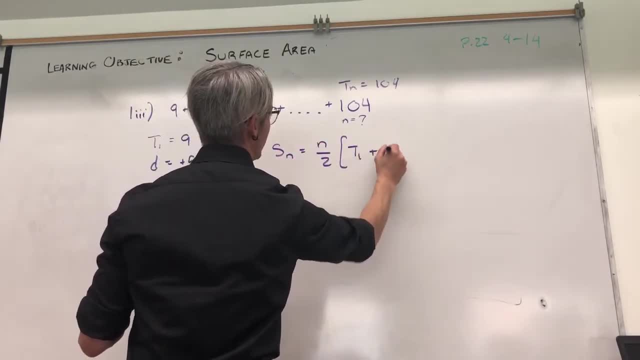 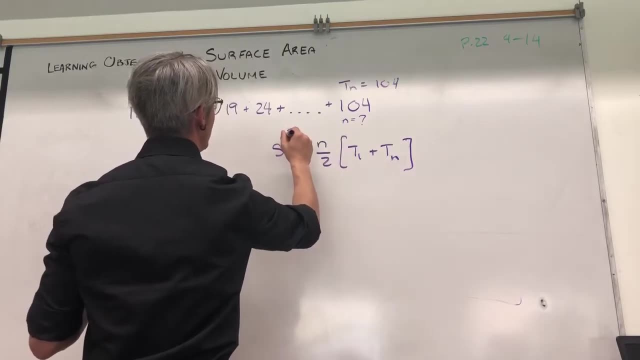 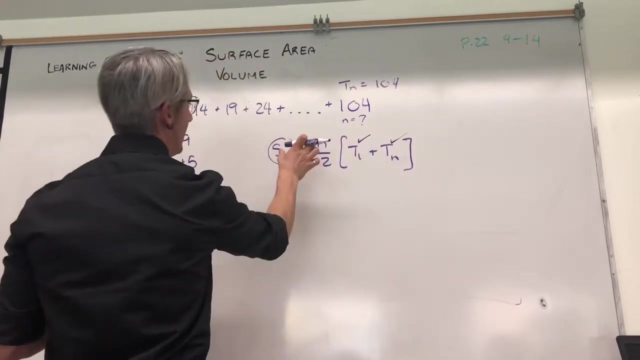 to N divided by 2. T1 plus T8. Or sorry, TN. Okay, I don't know this. This is what I'm trying to figure out. I don't know N, I know T1, and I know TN. I have two unknowns here. 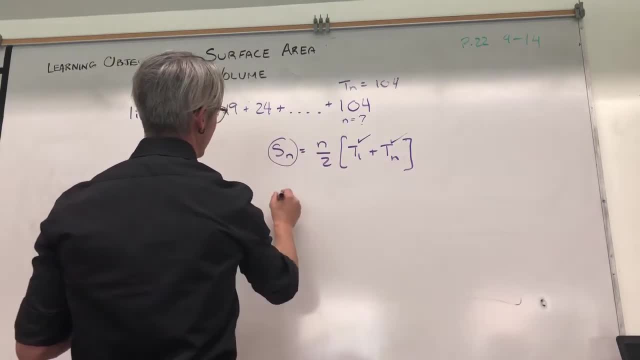 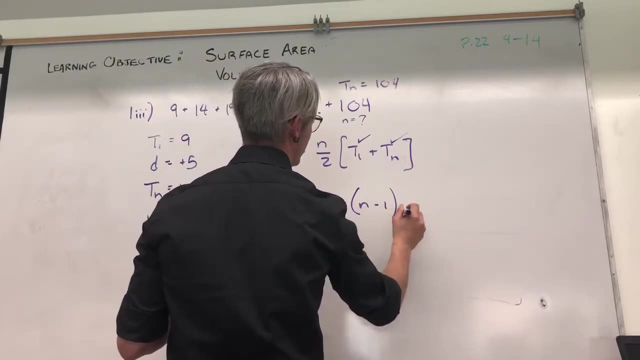 so I can't solve SN until I know what N is. So let's look at the other equation. I know T1 is equal to T1 plus N minus 1 times T. I know this, I know this and I know this. 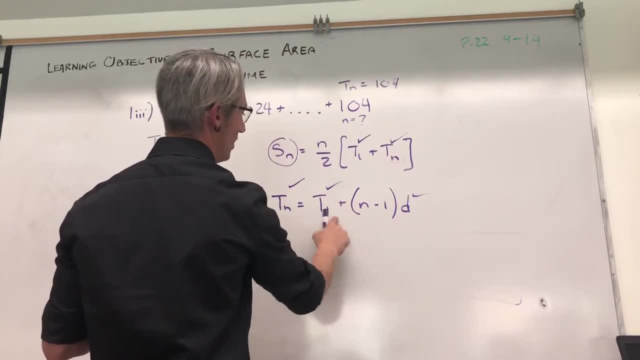 So I can solve for N. So let's solve for N. First off, T1, it's not married to anything, It's on its own. So I can subtract out T1 here. Actually, first let's put in the numbers. 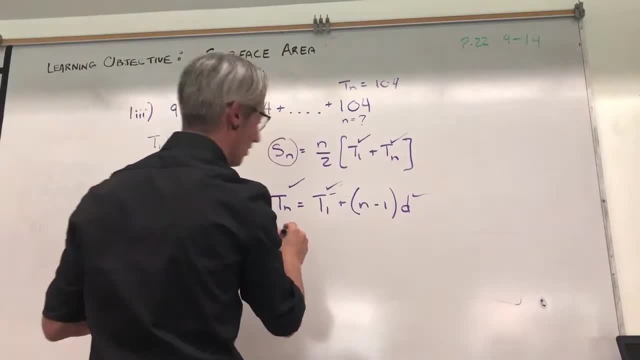 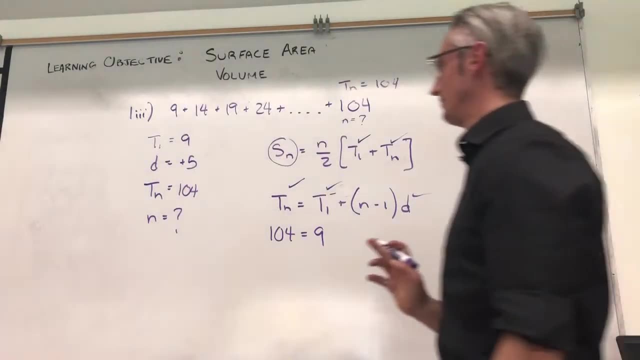 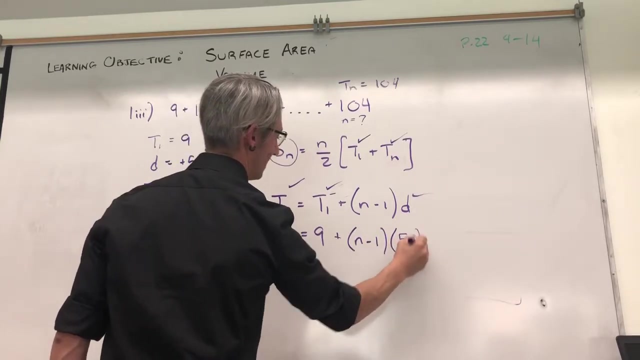 so I don't confuse you. So I'll put in: 104 is equal to 9.. Let me just make sure you can see all the numbers there. Okay, It's equal to 9 plus N minus 1 times 5.. Okay, So I can subtract out the 9 here because it's unattached. So 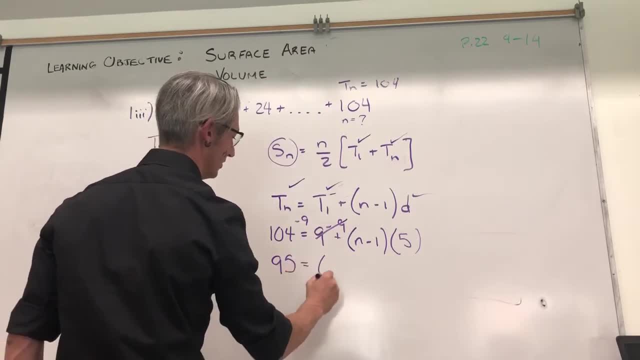 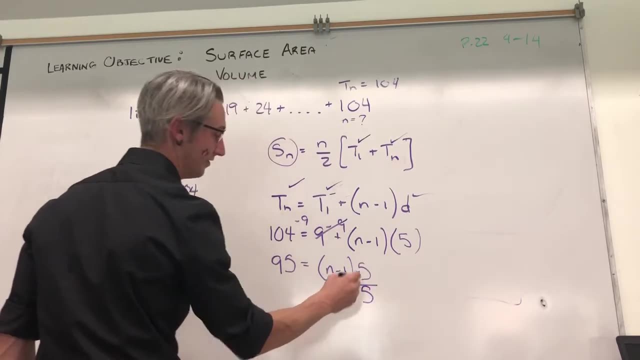 I'll have to do that. This becomes: 95 is equal to N minus 1 times 5 times. So I can subtract out, I can divide out the 5. What I do to one side, I have to do to the other. This. 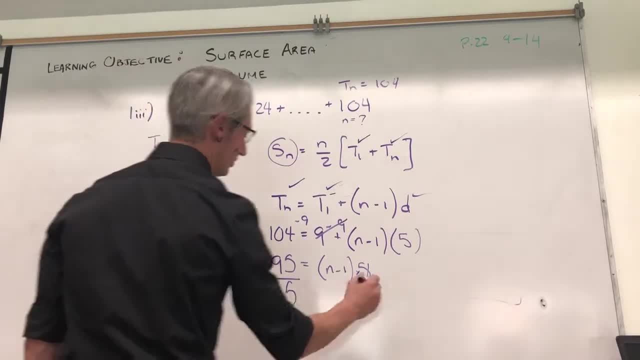 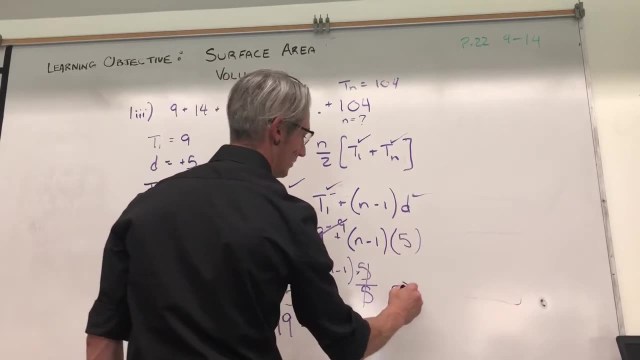 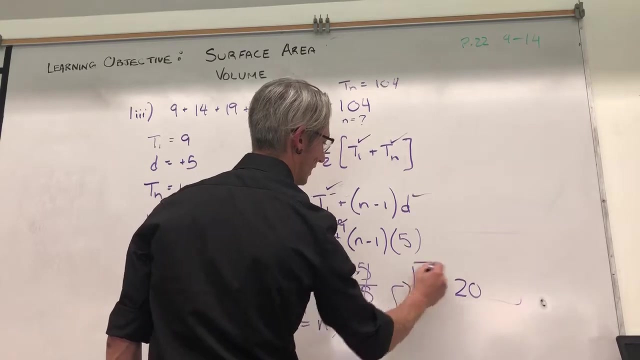 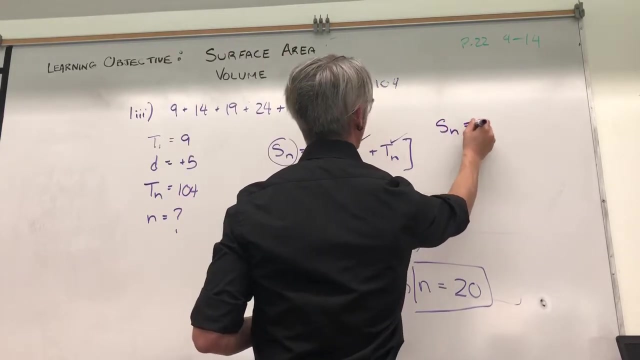 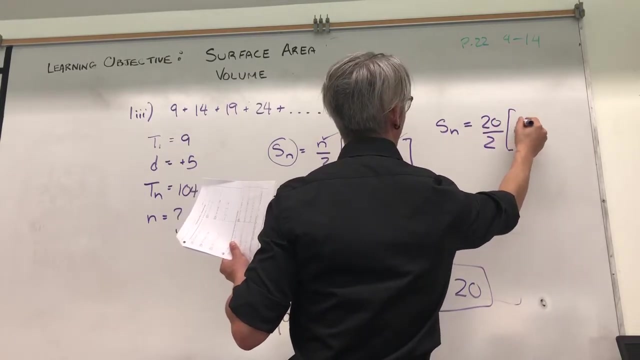 becomes 19.. So 19 is equal to N minus 1.. So N, and I add the 1 on each side, N, is equal to 20.. Okay, Now I have all that and I can solve for Sn. So Sn is equal to 20 divided by 2.. 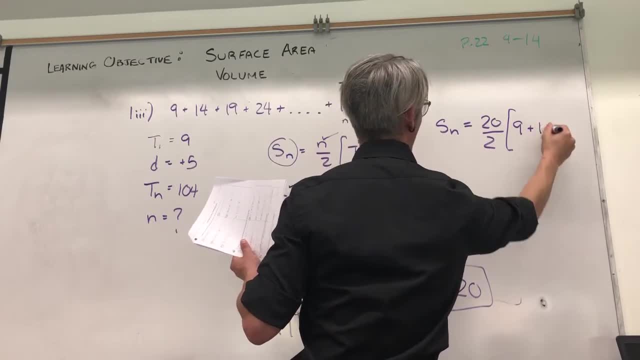 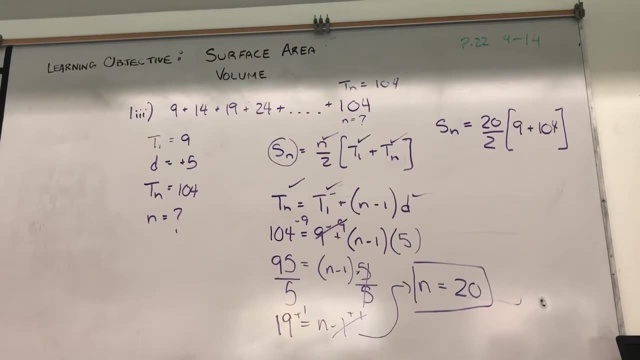 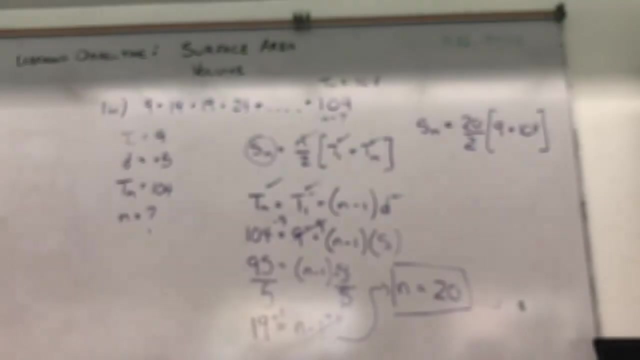 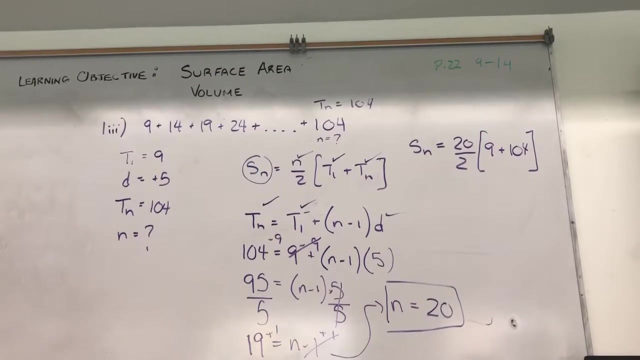 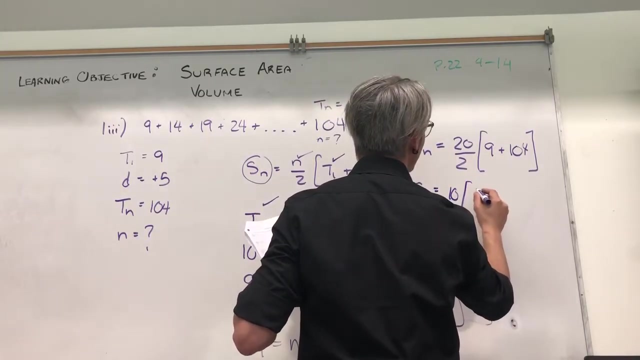 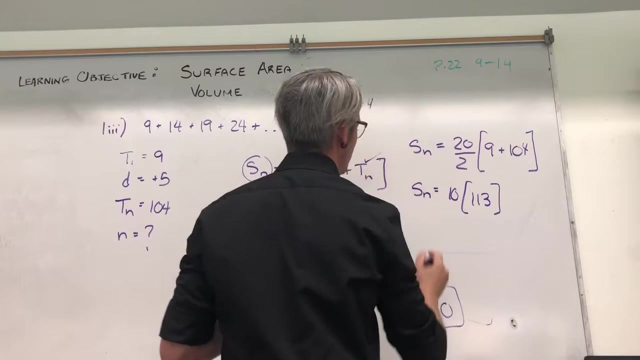 9. plus 104.. Let's make sure this is in the shot. Oh, it's in the shot. Okay, sorry about that. So 104 Sn is equal to 10 times 9 plus 104 is 113.. Sn is 1130.. 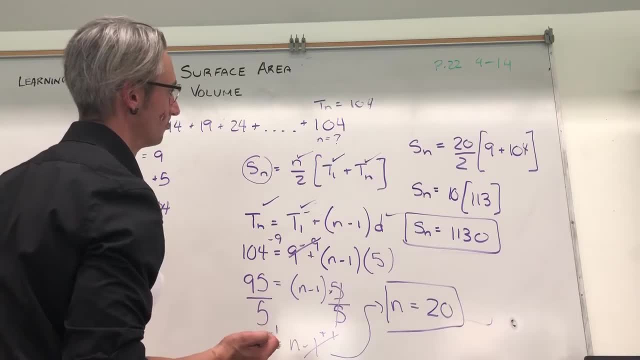 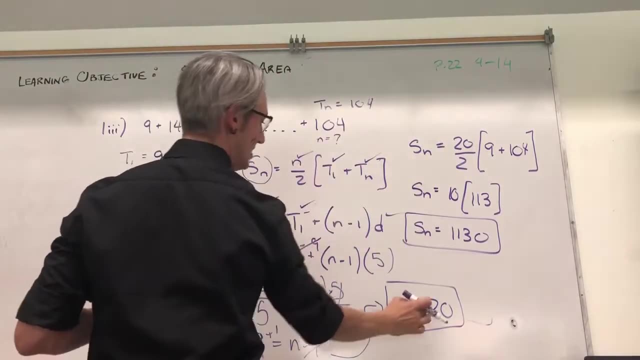 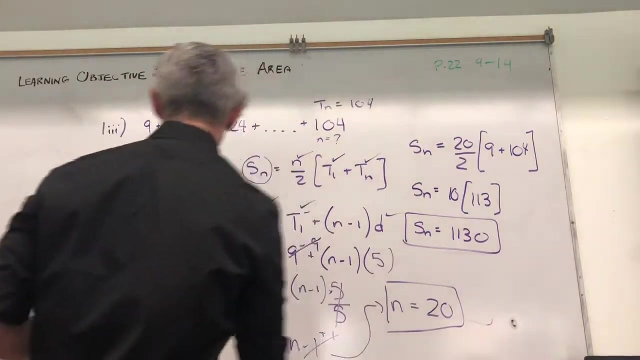 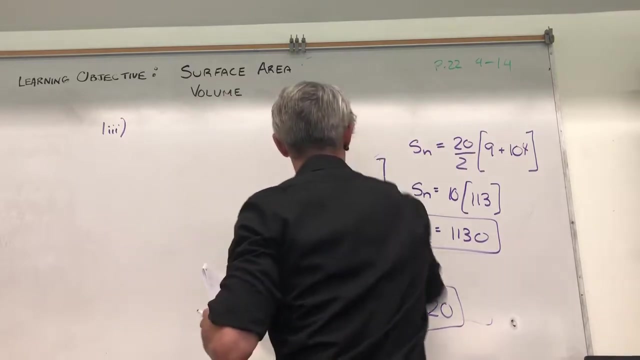 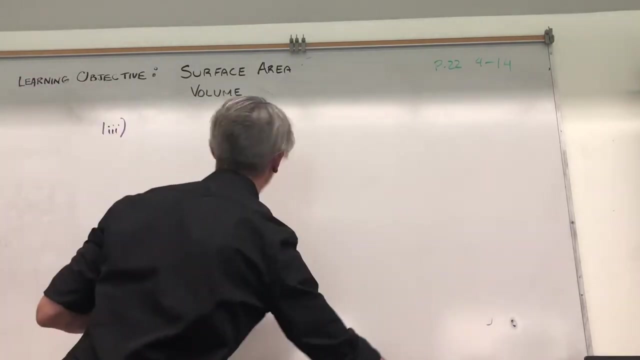 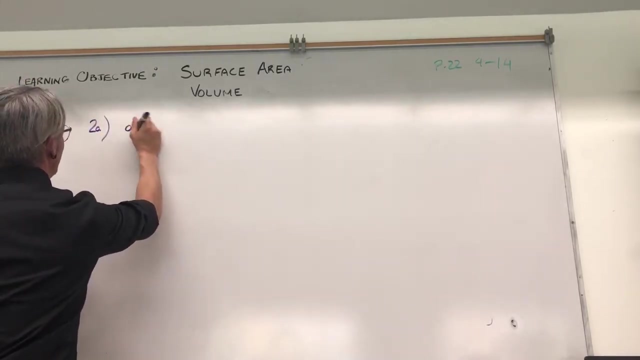 I hope I think so. Okay, so the sum of my 20 term series is 1130.. The last term is 104.. Okay, so let's do 2a. Okay, 2a, where a, which is the same as t1, is 12.. 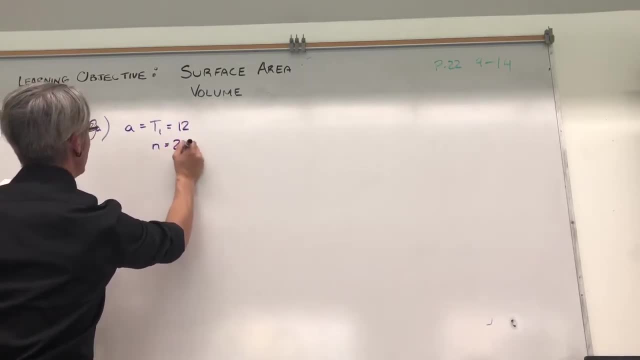 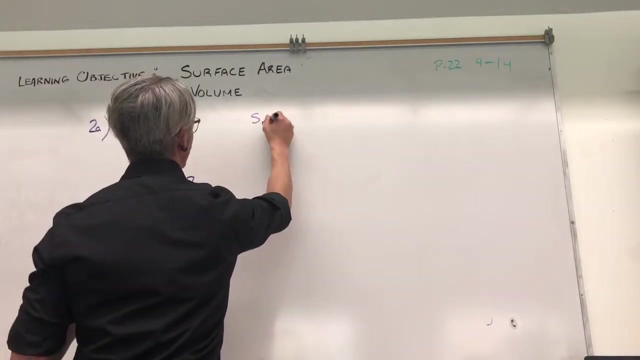 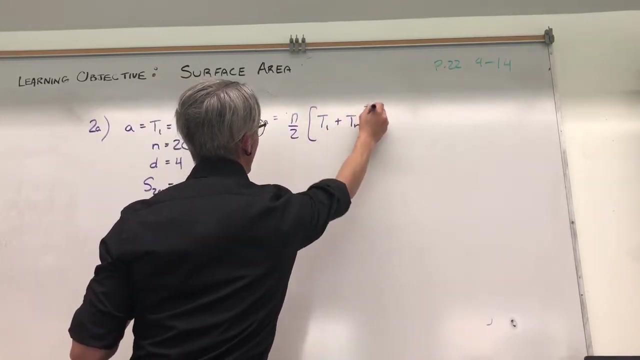 They tell us n is 20,, d is 4.. And they want to know what the sum of 20 terms, the first 20 terms of that series, is. Okay, so I go to my equation. Well, Sn is equal to n divided by 2 t1 plus tn. 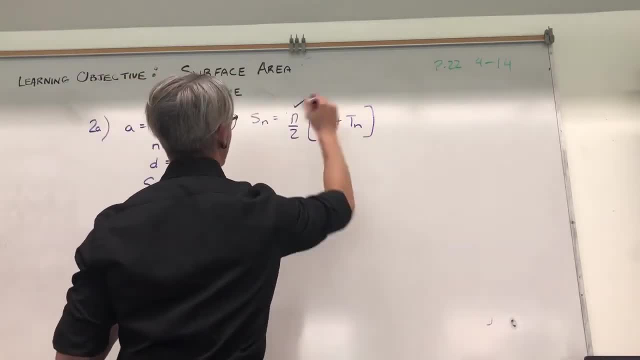 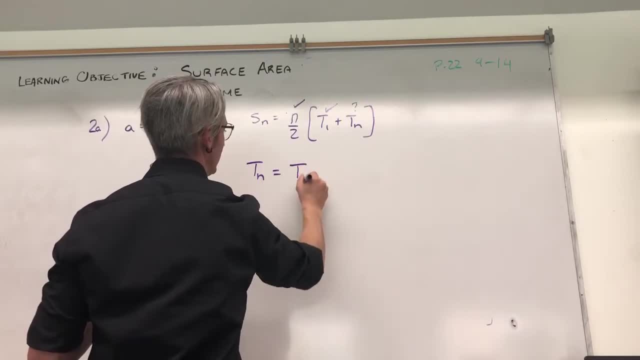 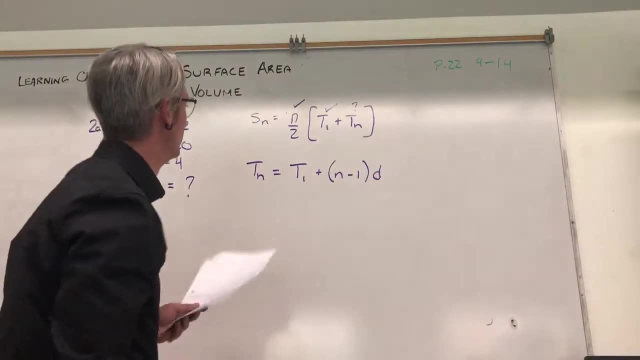 But I do have a formula for tn. My other formula: t1 plus n minus 1 times t. Okay, so I know this, I know this And I know this Easy peasy lemon squeezy, I can solve this. 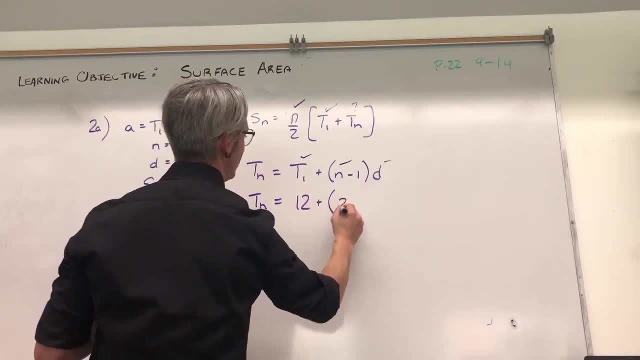 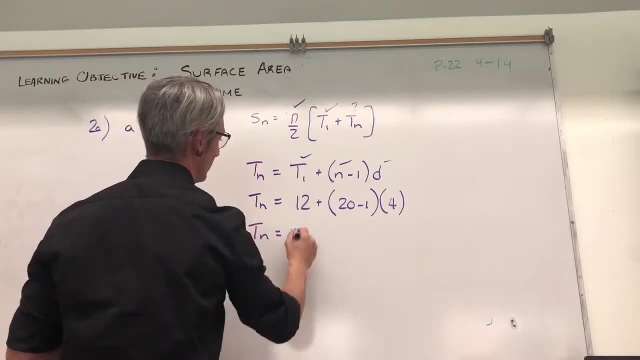 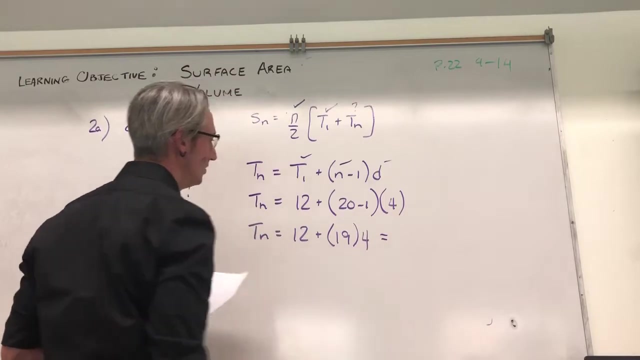 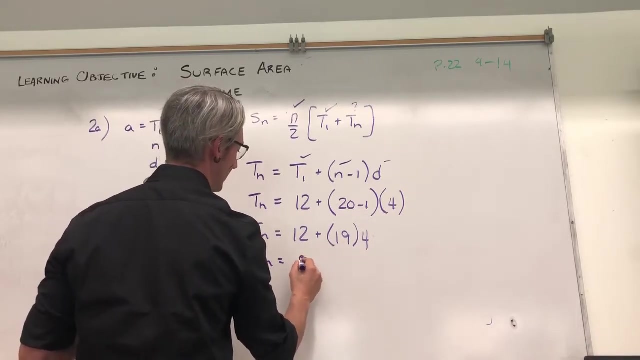 t1 is 12.. 20 minus 1 times 4.. tn- tn becomes 12 plus 19 times 4,, which is equal to tn, is equal to 19 times 4 is 76, 88.. Okay, now I can take this back into here. 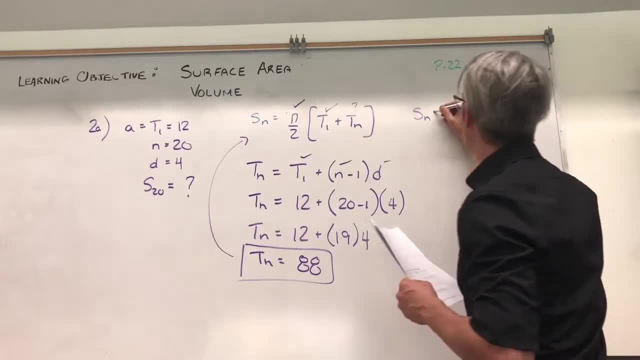 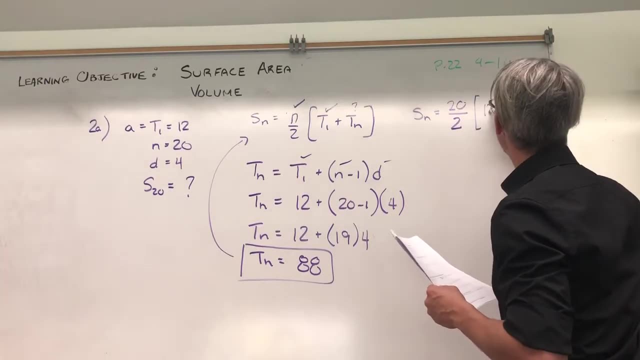 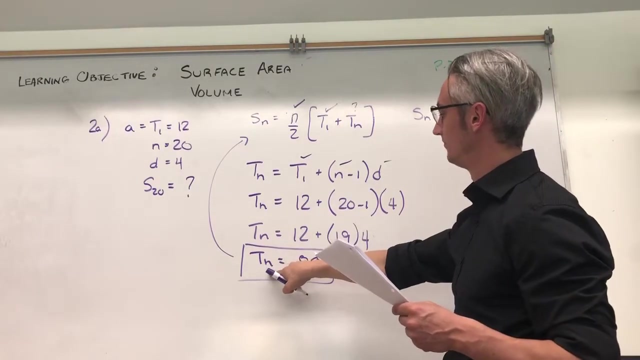 So now, Sn equals 20 divided by 2. 12 plus 88. My 20th term, tn, my last term, when n is equal to 20.. So tn is the same as t when n is equal to 20, which is 88. 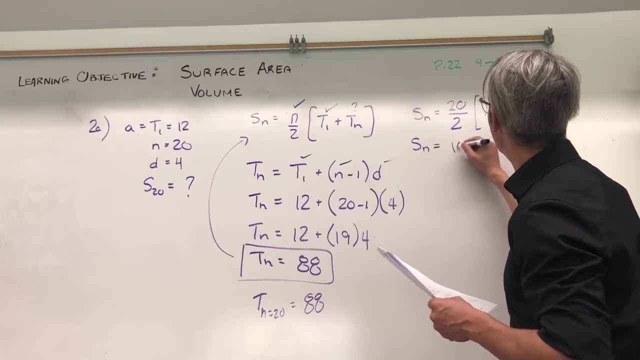 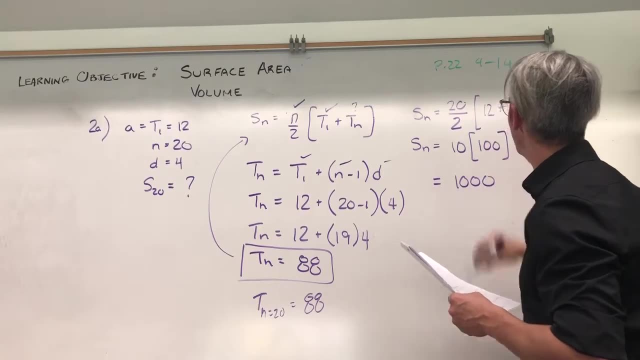 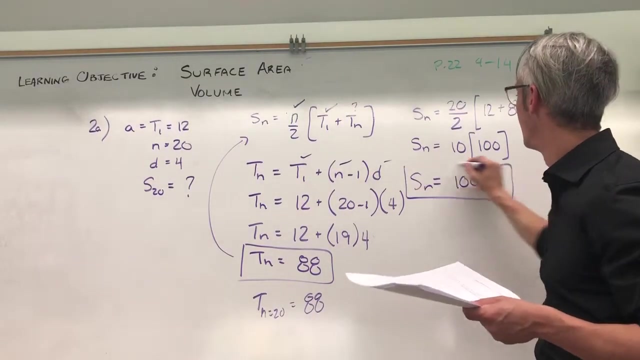 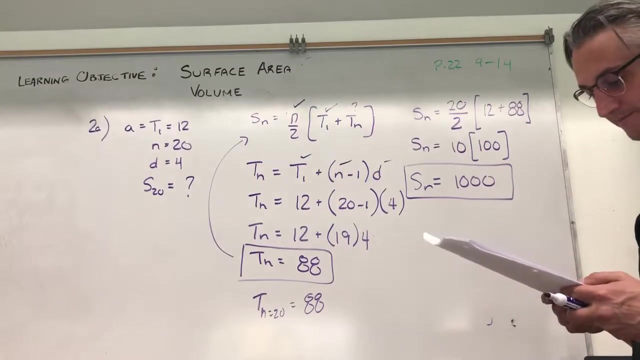 So this becomes: Sn is equal to 10 times 100 is equal to 1000.. I hope I might be making mistakes. Maybe you'll catch them. Okay, not so bad. Okay, let's try a hard one. Let's try 2e. 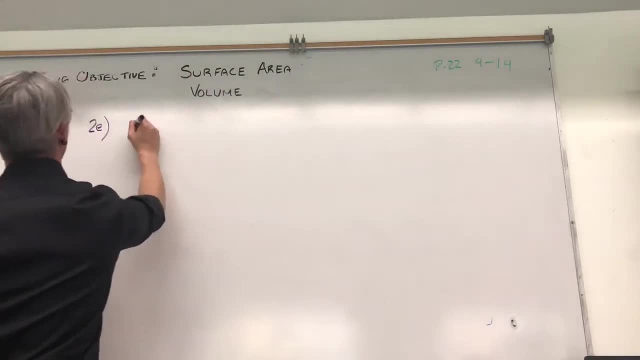 2e, where they tell me that t1 or a is 12.. The sum of first 15 terms is 453.. And they want to know what d is equal to. Well, I also know that n in this case is going to be 15, because we're dealing with the first. 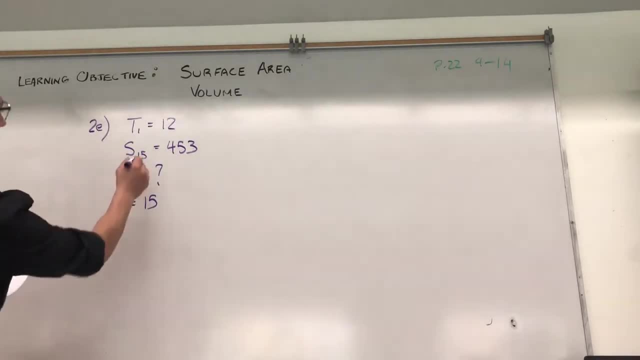 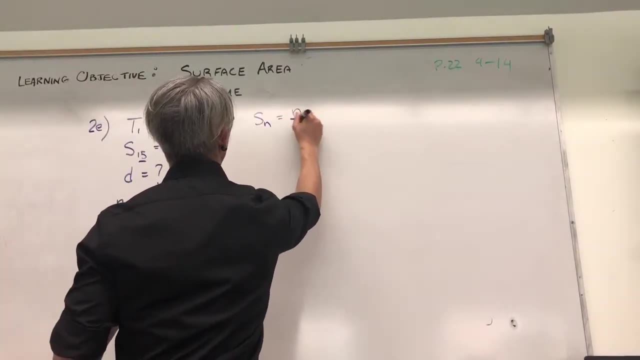 15 terms. So n is 50.. I took that from right here kind of like a little sneaky thing they do to us. So I go to my equations. Sn is equal to n divided by 1.. Sn is equal to n divided by 2.. 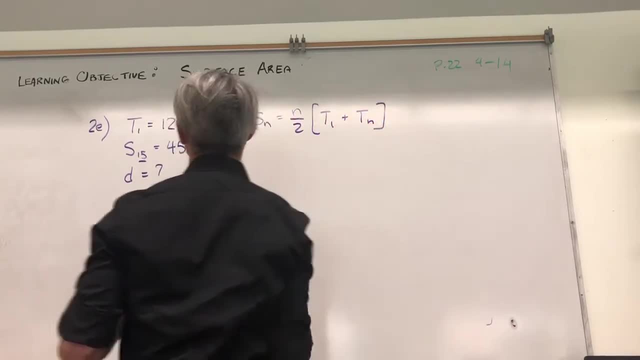 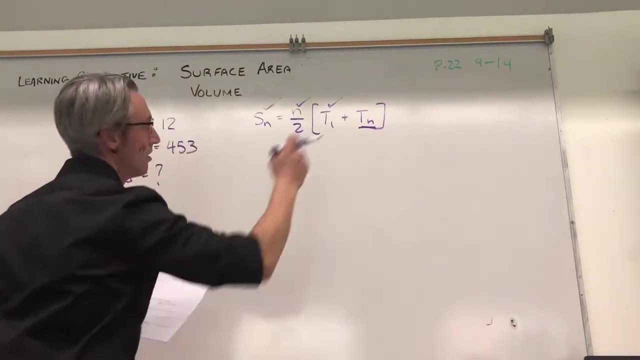 t1 plus tn. I know this, I know this and I know this, So I can actually solve for this And I'm probably going to use that in the next equation to solve for d. So let's solve for that right now. 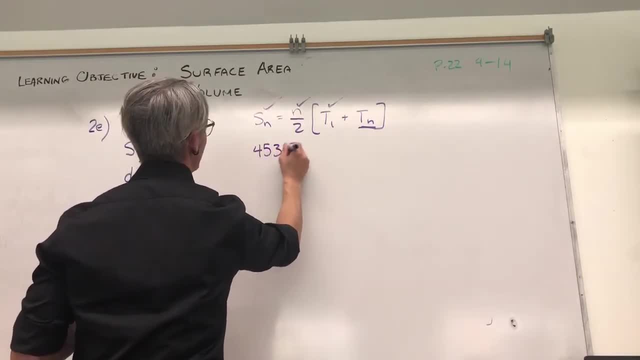 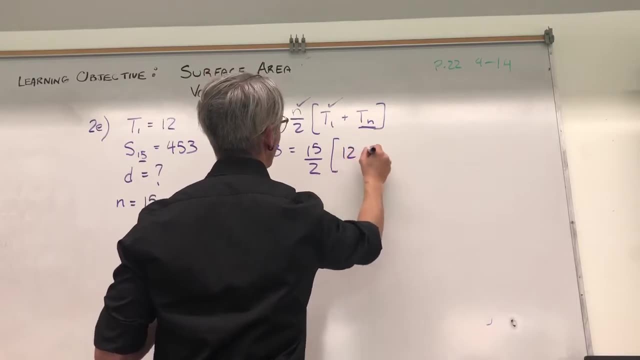 Well, so let's plug. stuff in: 453 is equal to 15 divided by 2.. 12 plus t1.. Let's plug. stuff in: 453 is equal to 15 divided by 2.. 12 plus t1.. 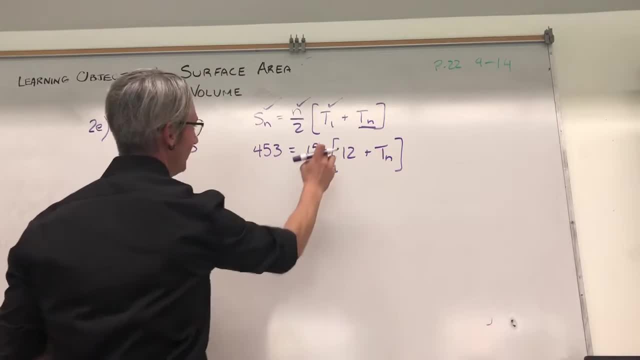 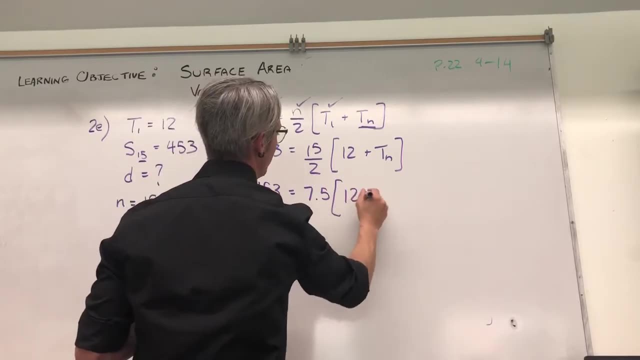 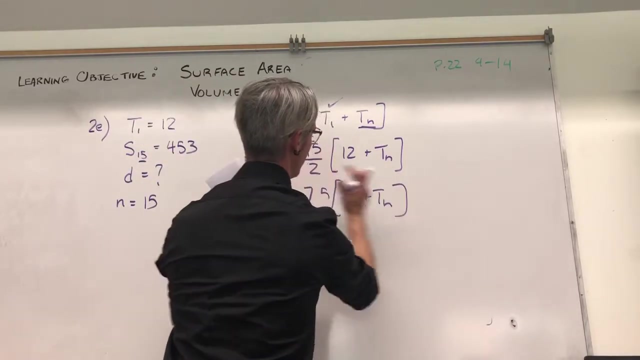 This is 7 and a half. Well, let's rewrite it: 453 is equal to 7.512 plus tn. Now I can't play around with this, because this is a family. It's in the bracket, So it's together right now. 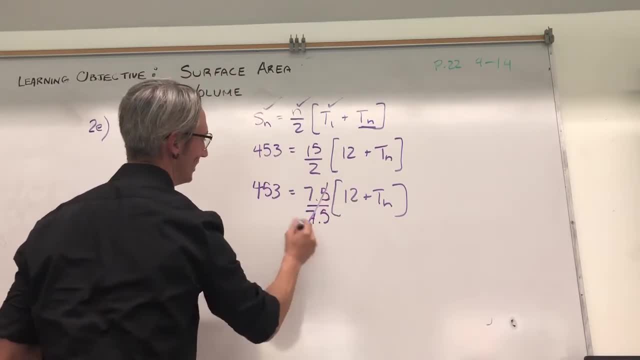 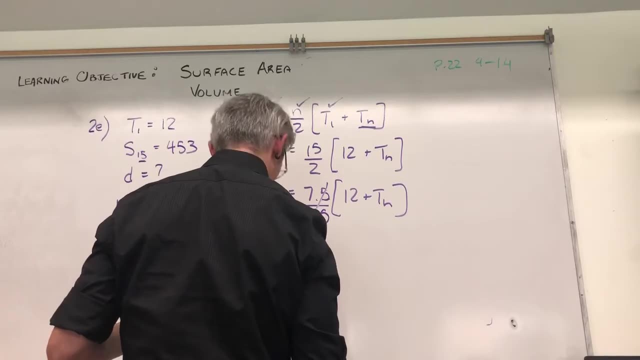 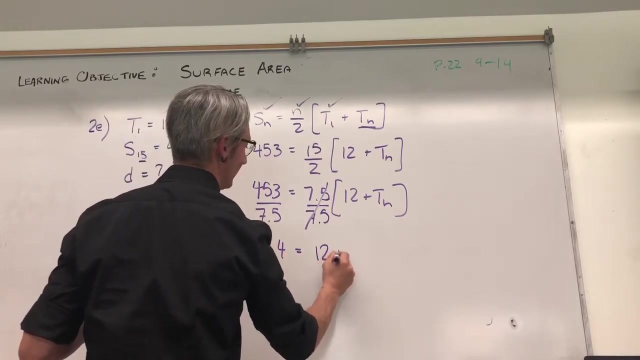 But I can. The 7.5 is on the outside being multiplied, So I can do the opposite. That becomes 1. 453 divided by 7.5.. 60.4.. So 60.4 is equal to 12 plus tn. 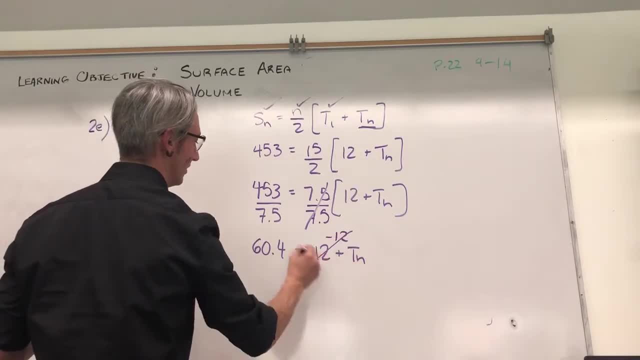 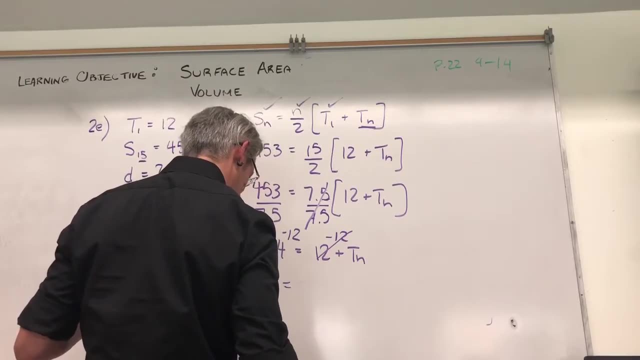 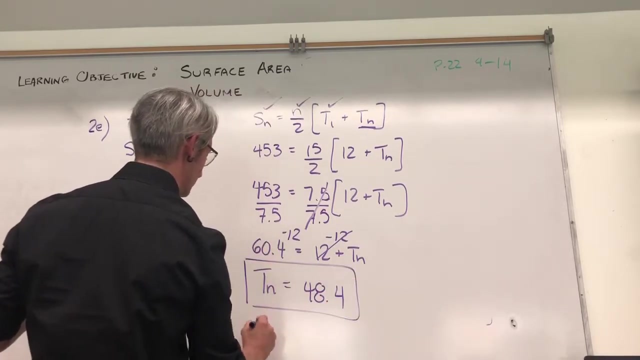 Now it's easy for me to get rid of this 12 here, Which I do to both sides, And I find out that tn is equal to 60.4 minus 12. 48.4.. That is my value when n is equal to 1.. 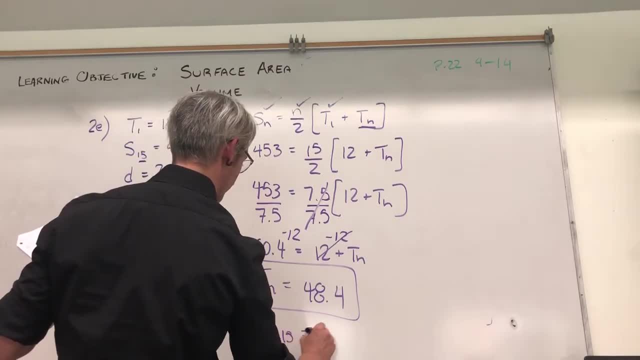 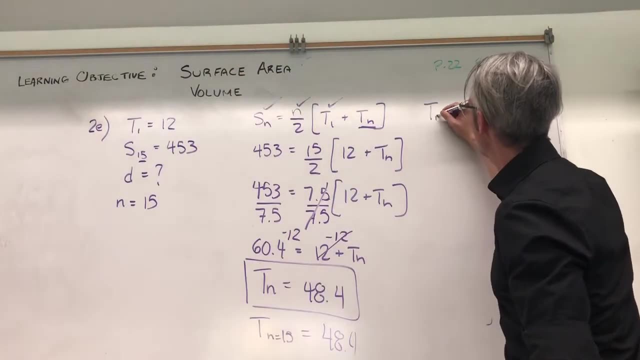 That's my 15th term, 48.4.. Okay, So now let me use my equation for tn to figure out d. So tn is equal to t1 plus n minus 1 times d. Now I'm solving for d.